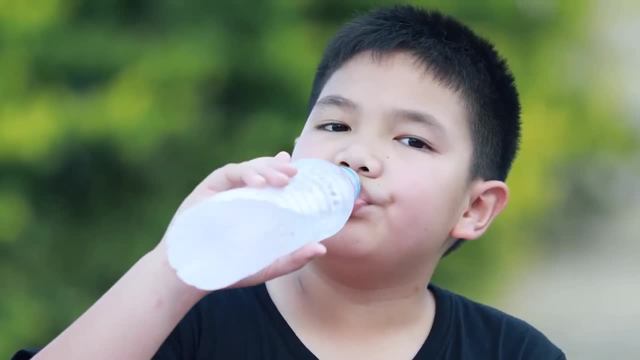 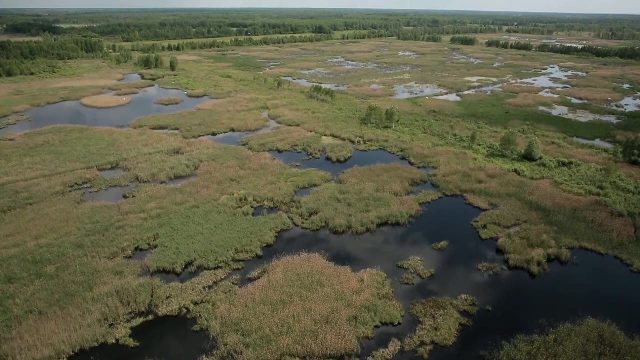 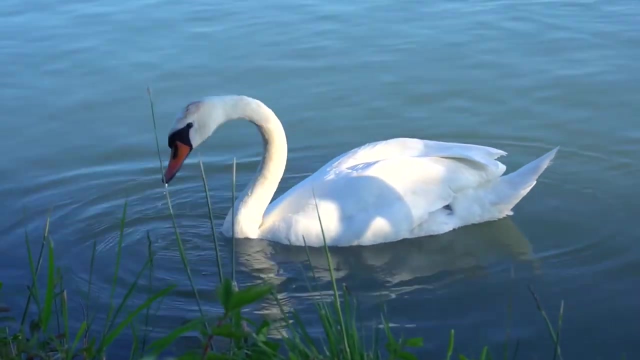 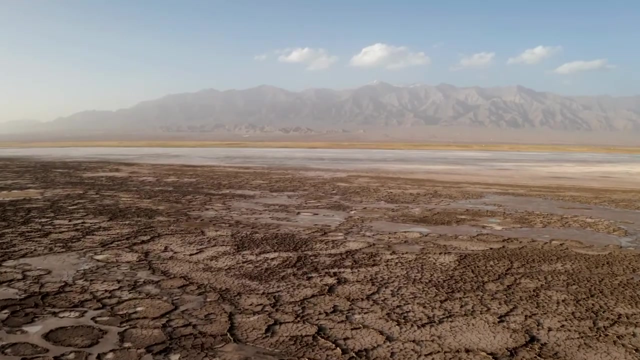 to consume water daily to maintain our body functions. for plants, water is necessary for growth, photosynthesis and nutrient absorption. animals depend on fresh water for hydration, habitat and sustenance. without fresh water, ecosystems would crumble and life as we know it would cease to exist. importance of fresh water for biodiversity. 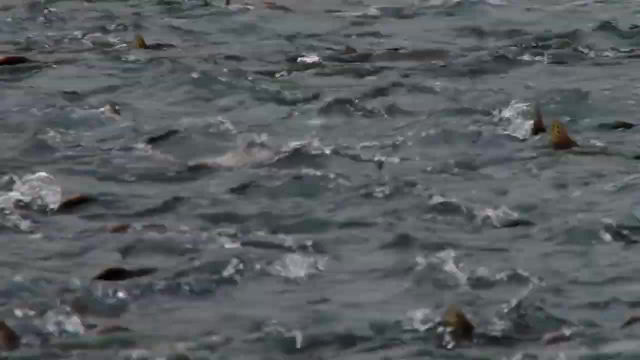 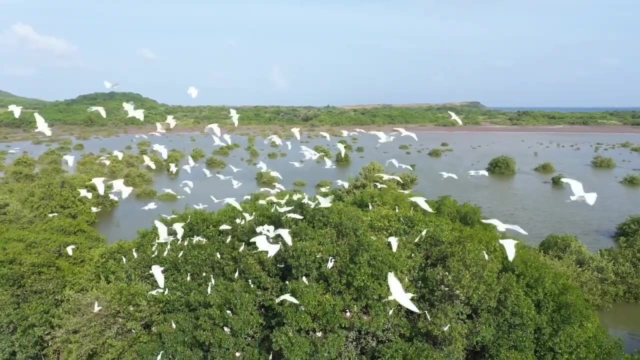 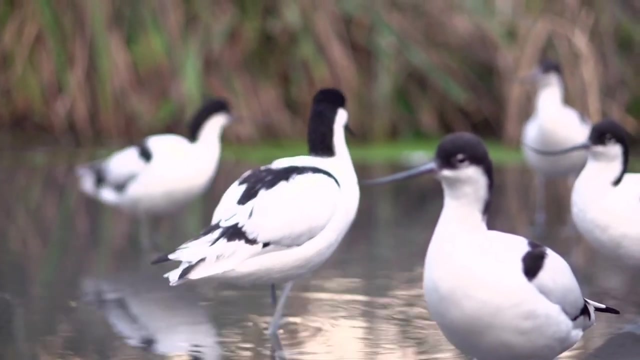 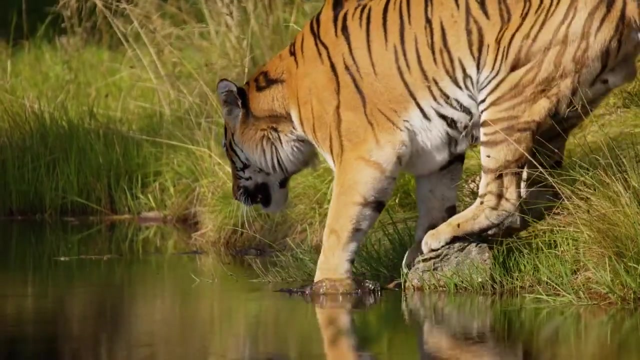 fresh water habitats such as rivers, lakes and wetlands support a wide array of species. these habitats are critical for maintaining global biodiversity as they provide unique environments for many specialized plants and animals. the high species risk of natural disasters and water np's then produce the environmental impact of fresh water around living organisms. 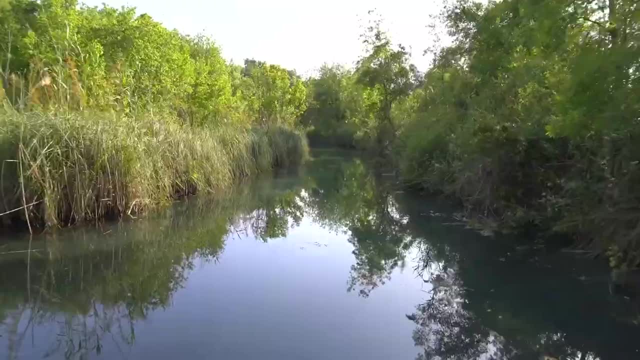 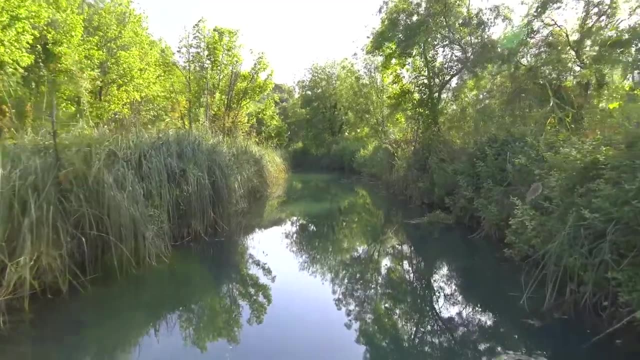 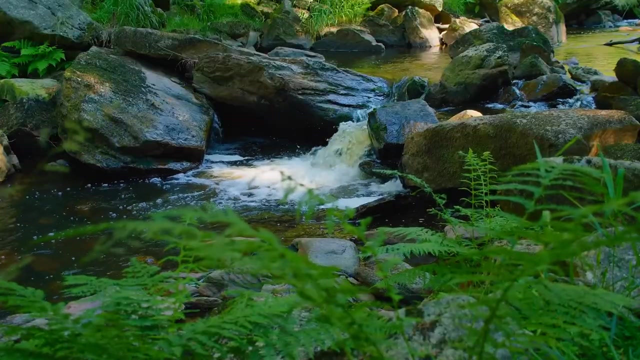 these ecosystems at the need for child born faunaights. their 제대로 usually build a high�ases as human excrement. life can increase and the answer to that is very uncertain for species. each species may be family if they are unified or belongs to a different species form. SAP, Anthem, grandfather pr dementia body is an energetic. 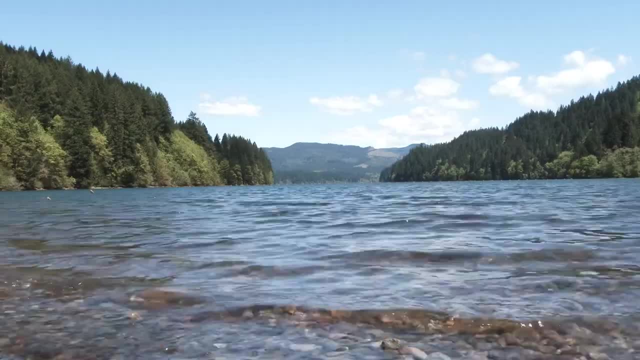 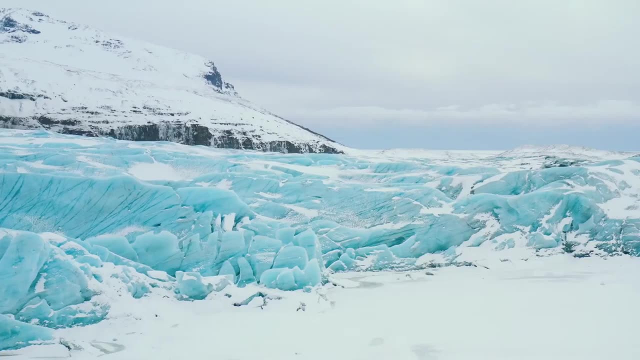 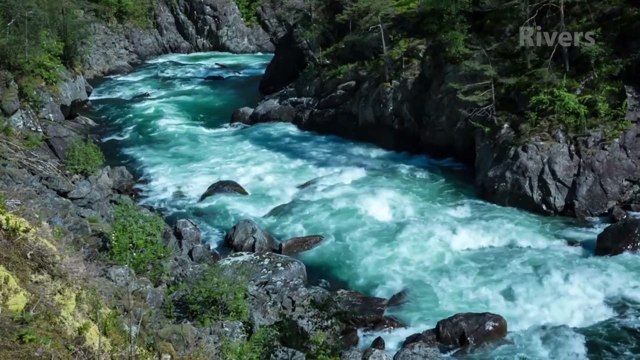 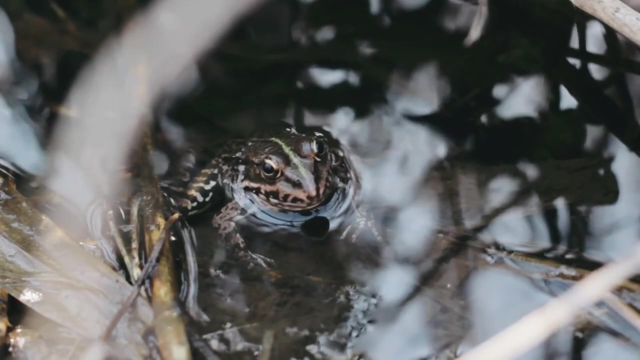 Surface water includes lakes, rivers and wetlands, while groundwater is the water stored beneath the Earth's surface in soil and rock formations. Ice, such as glaciers and ice caps, represents another significant source of freshwater Rivers. Rivers are considered open systems because they are continuously receiving and releasing water, nutrients and organisms. Human activities and natural processes can greatly impact river systems. For example, agricultural runoff can introduce pollutants and excess nutrients into rivers, leading to the growth of harmful algal blooms that deplete oxygen and threaten aquatic life. Deforestation can increase sedimentation in rivers, altering habitats and reducing water quality. 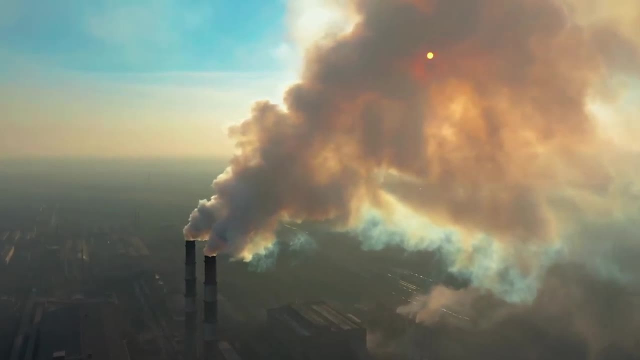 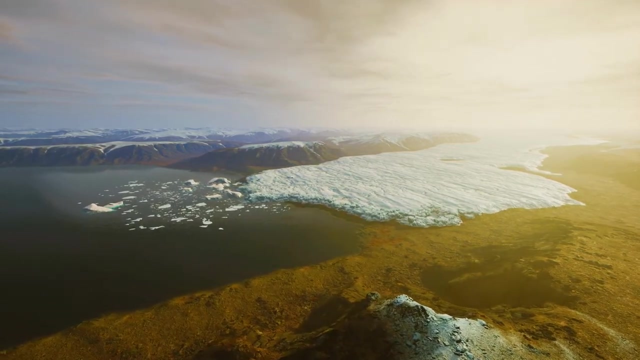 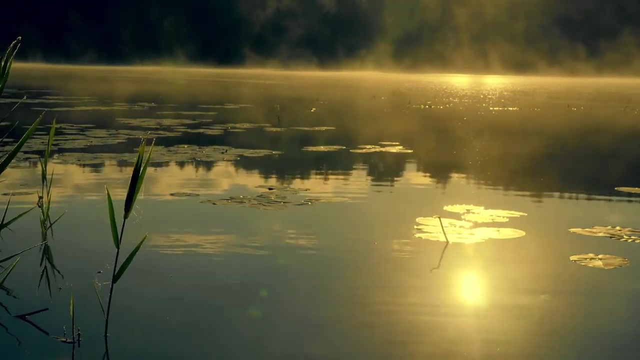 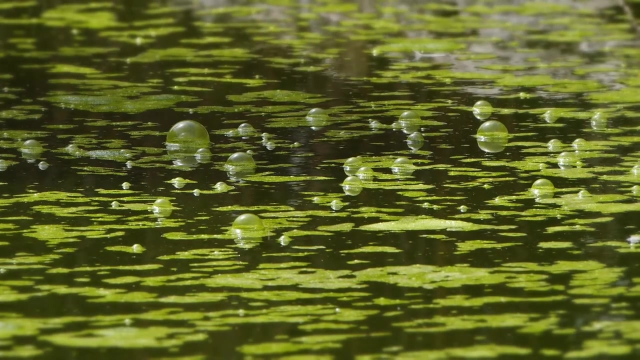 Climate change can also affect river systems, causing shifts in temperature and precipitation patterns and altering water flow and availability. Ponds and lakes: Unlike rivers, ponds and lakes are considered closed systems. They have limited exchange with their surrounding environment, which makes them more susceptible to pollution and other impacts. 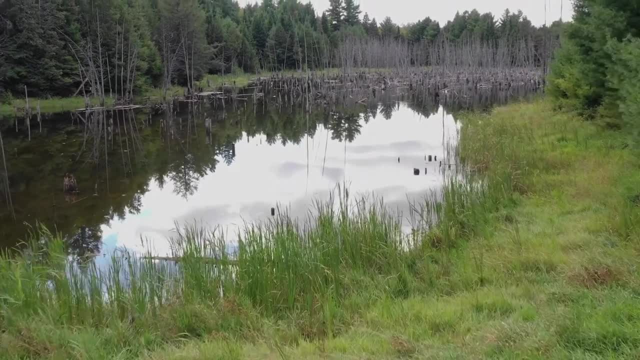 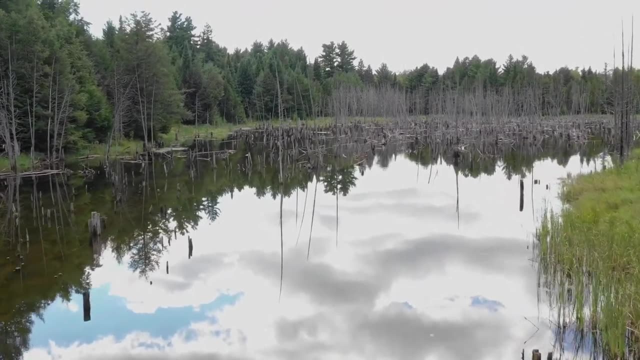 In closed systems, the water's chemical and physical properties are limited. In closed systems, the water's chemical and physical properties are limited, such as temperature. oxygen levels and nutrient concentrations remain relatively stable. However, human activities like nutrient loading from agricultural or urban runoff. 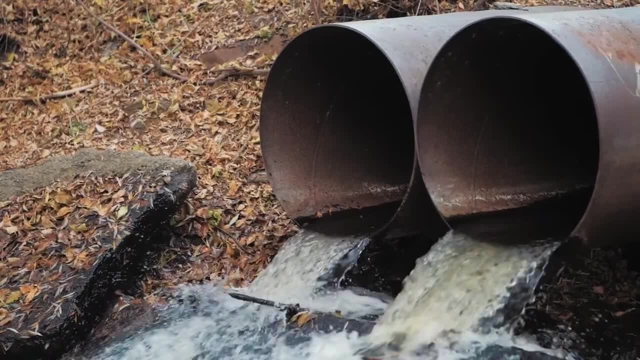 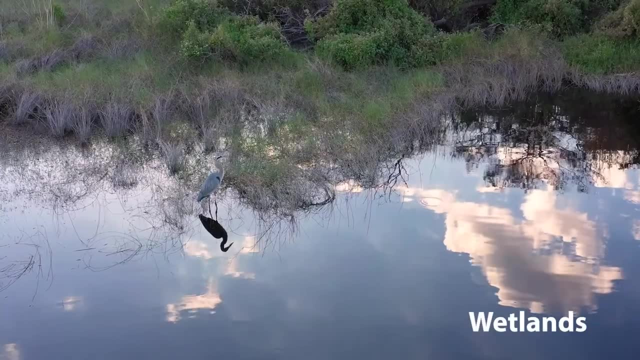 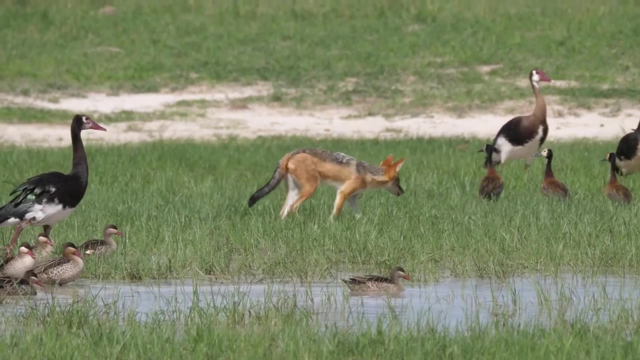 can disrupt the balance in these ecosystems, leading to issues such as eutrophication and loss of biodiversity. Wetlands- Wetlands are unique ecosystems where land and water meet, creating a diverse habitat for a wide range of species. They include marshes. 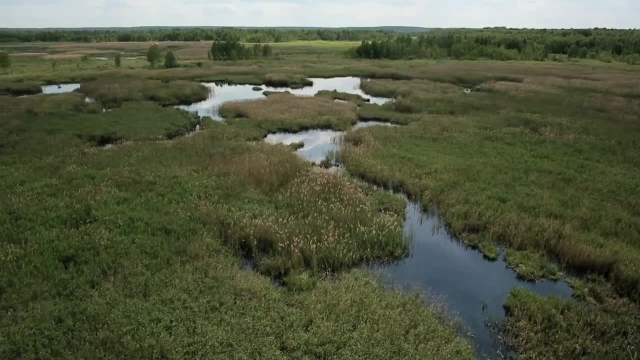 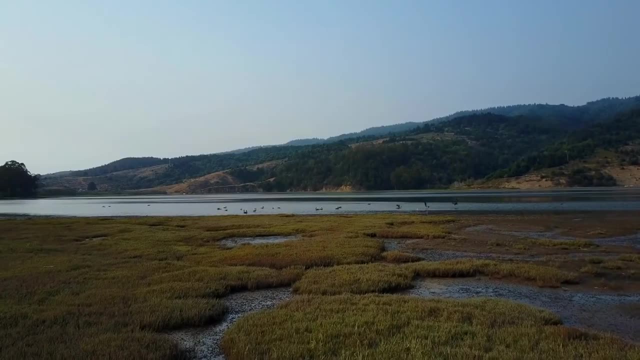 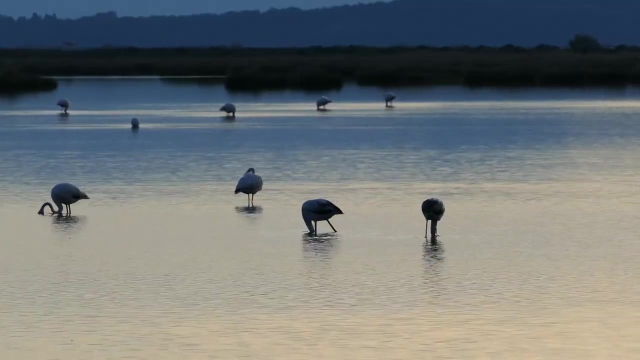 swamps, bogs and fens. Wetlands play a critical role in maintaining water quality, as they act as natural filters, absorbing pollutants and nutrients from the water. They also provide essential flood protection by absorbing and storing excess water during periods of heavy rainfall. 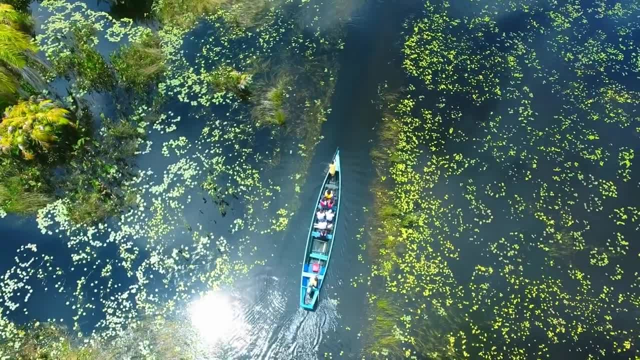 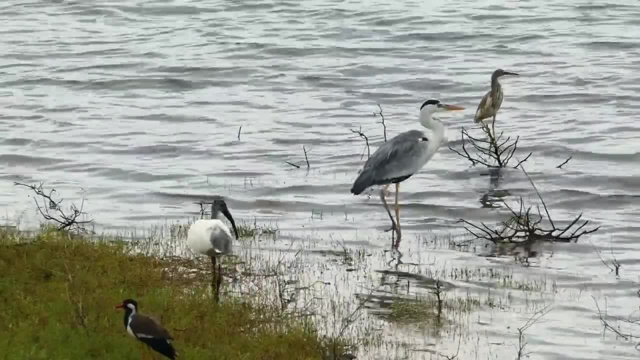 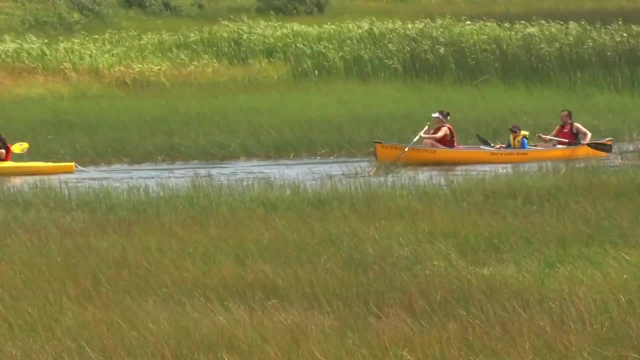 In addition to their ecological benefits, wetlands offer numerous cultural, recreational and economic values. They serve as vital habitats for many migratory bird species, support commercial and recreational fisheries and provide opportunities for ecotourism. The protection and restoration of wetlands are essential for maintaining the health of 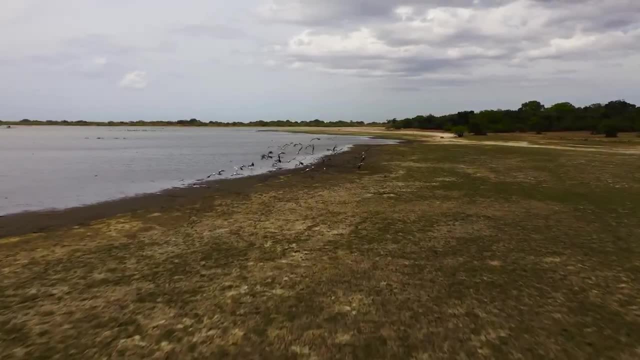 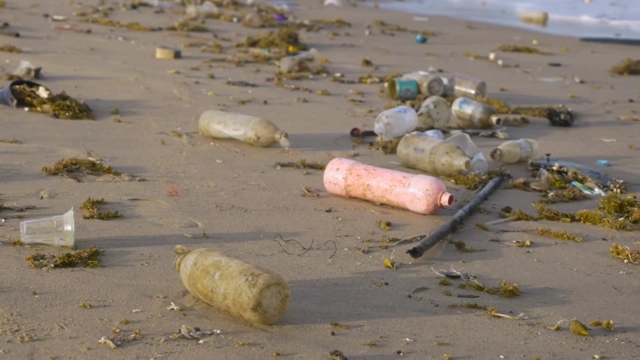 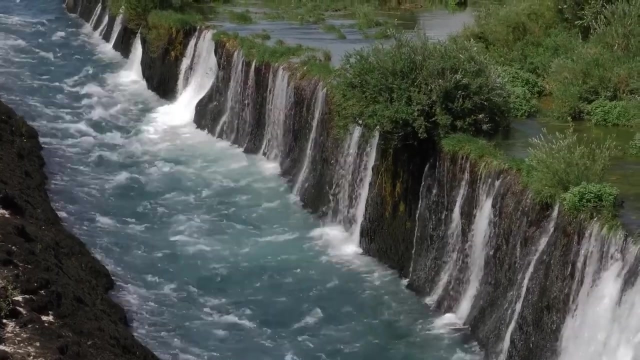 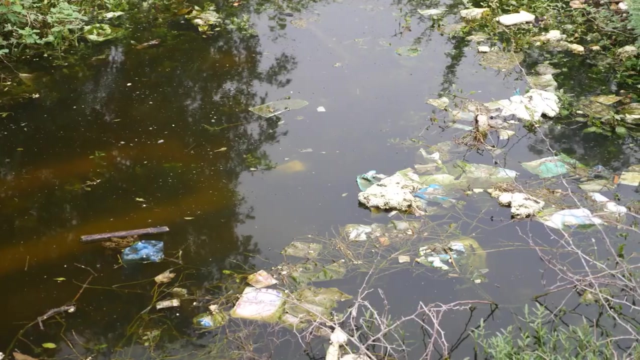 our planet and the well-being of future generations. Human Impacts on Freshwater Sources. Human activities have significantly impacted freshwater sources, leading to issues like pollution, changes to land and alterations to the natural flow of freshwater through the construction of dams. Pollution is one of the major threats to freshwater sources. 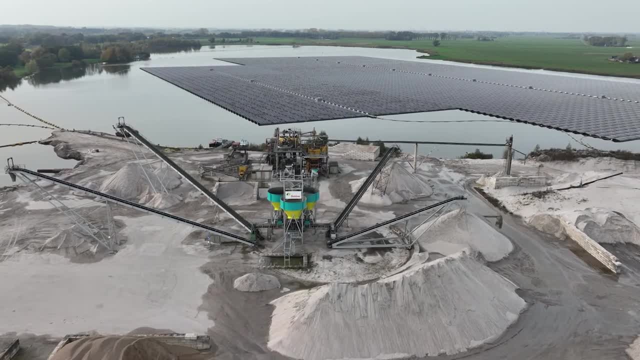 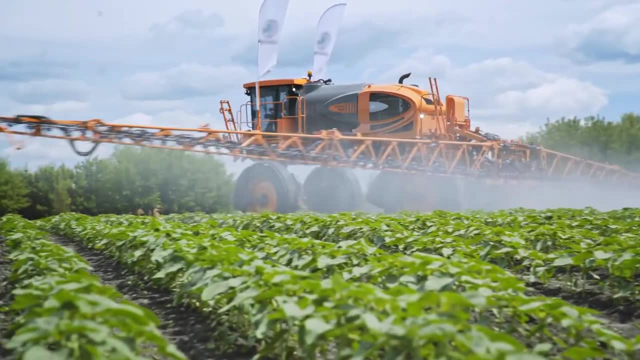 Agricultural, industrial and urban activities can introduce pollutants such as chemicals, heavy metals and organic waste into water bodies. Pesticides and fertilizers can also be used to produce pollutants, and fertilizers used in agriculture can leach into groundwater or be carried by runoff into. 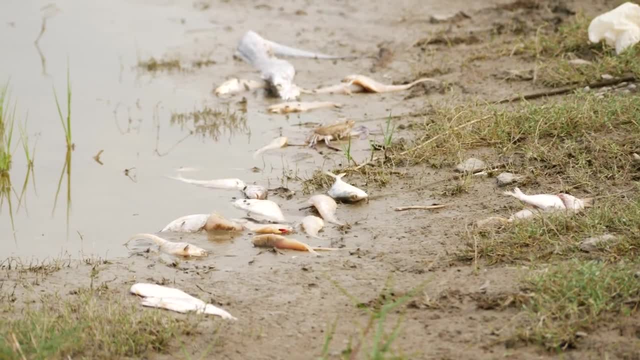 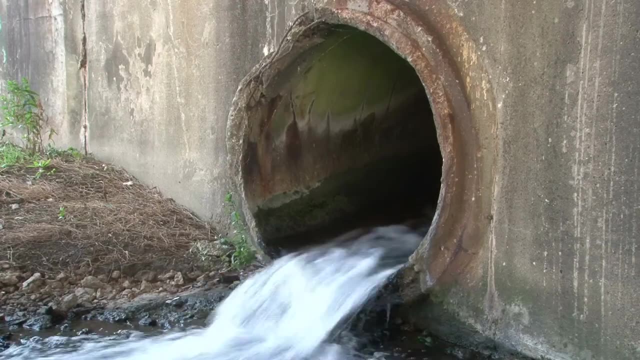 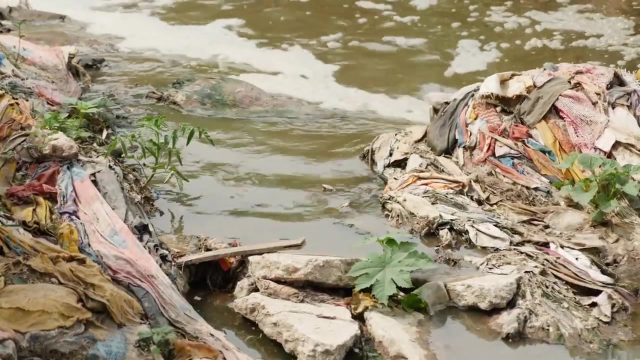 rivers and lakes, causing harm to aquatic life and affecting water quality. Industrial discharges, untreated sewage and litter can also degrade freshwater ecosystems, posing risks to both human health and the environment. Human-induced changes to land, such as deforestation, urbanization and agroecology, can also be.